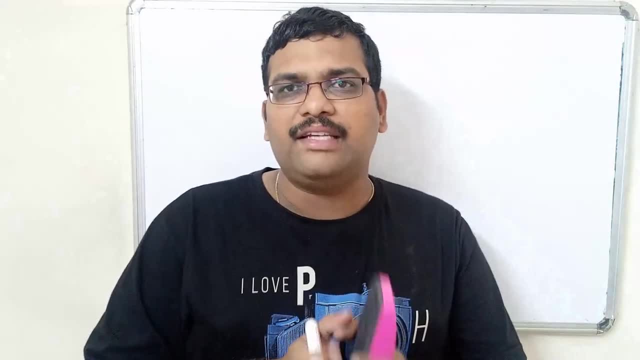 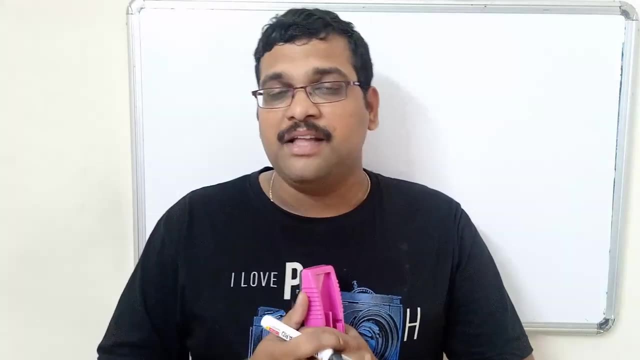 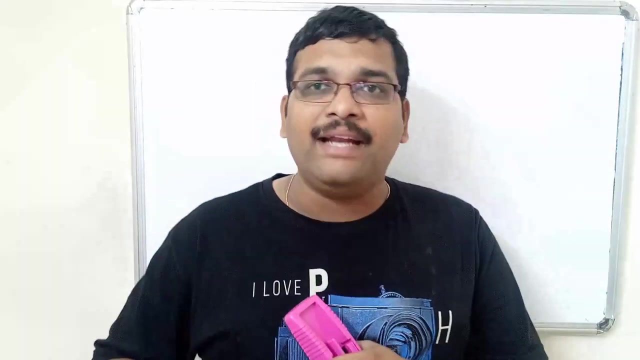 So frequently asked. a question in every written test is on a calendar problem. right, We can expect one question on calendar problem. That means finding the particular day of given date. So now in this session, let us check how to find the day, if the date is given right, See? 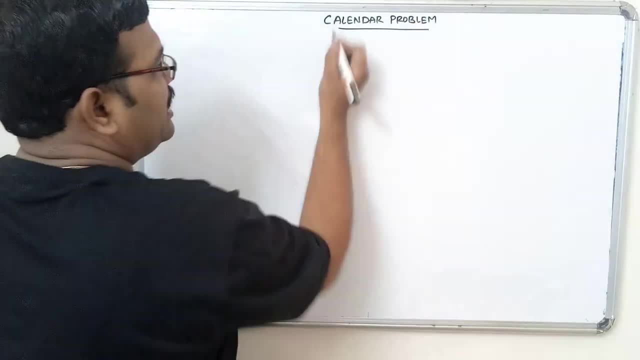 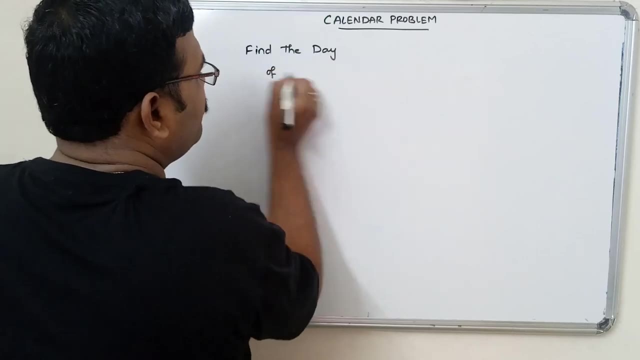 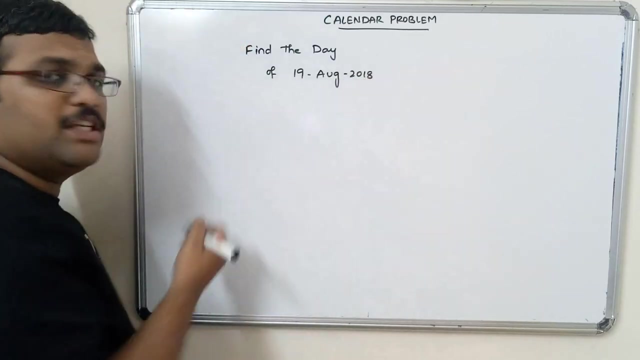 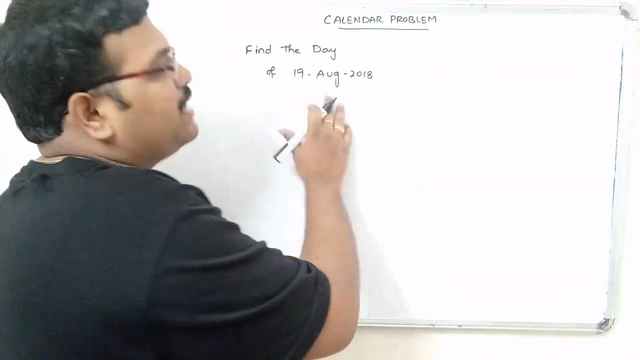 Calendar problem. So the question is: find the day of 19th August 2018.. Right, So obviously we know the answer: that is Sunday. Today itself, it's a 19th August 2018, right, If it is 19th August? 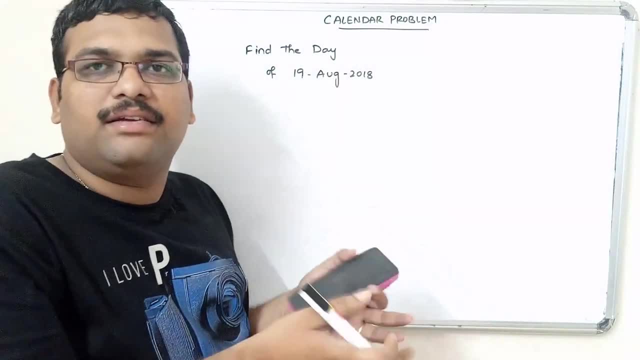 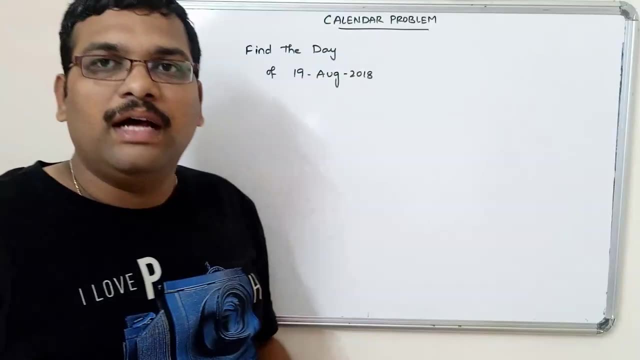 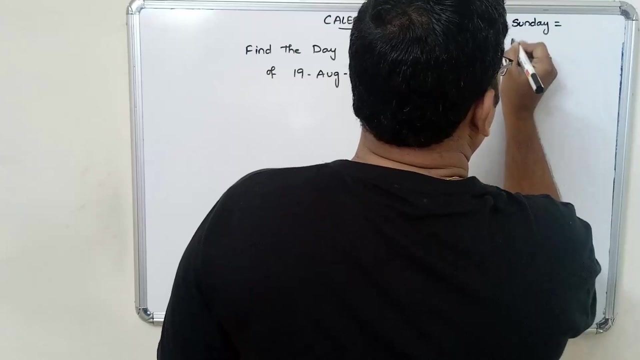 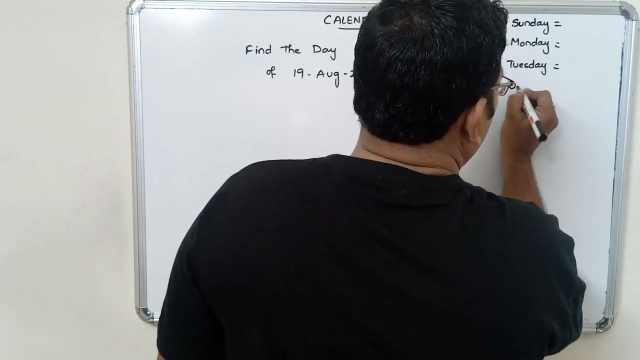 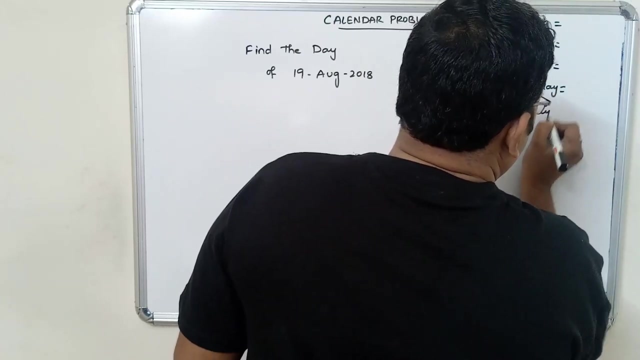 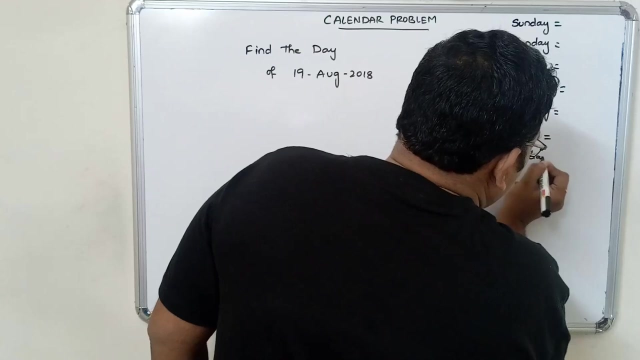 2000,. then it is difficult to calculate manually, right? So we need some shortcuts to find the day easy. So for this have to remember some codes first. take the codes for all the days: sunday, tuesday, wednesday, thursday, friday and saturday. 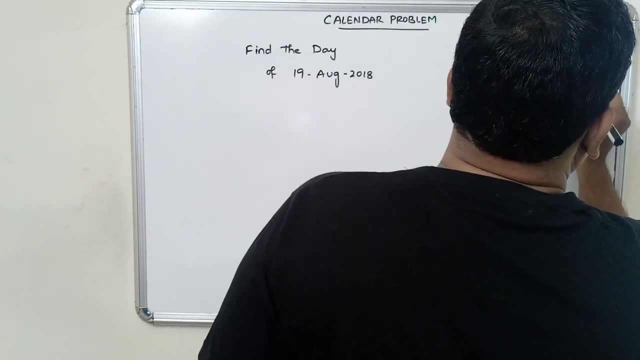 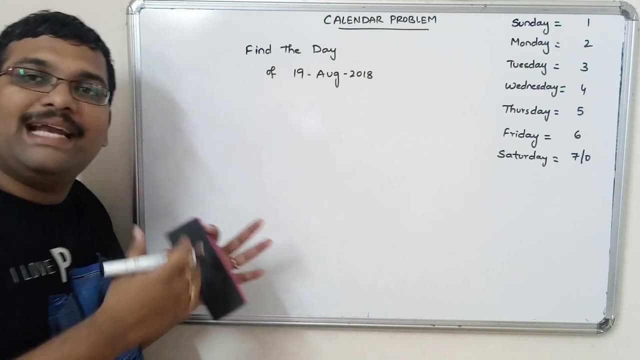 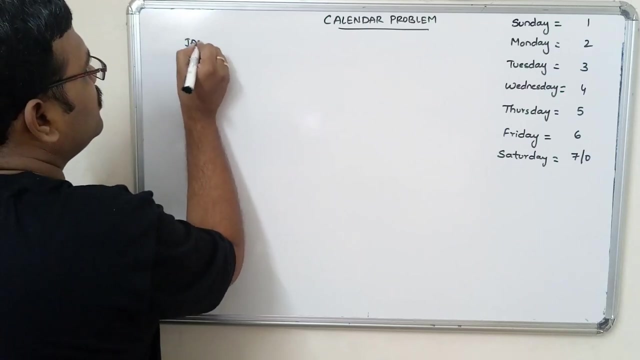 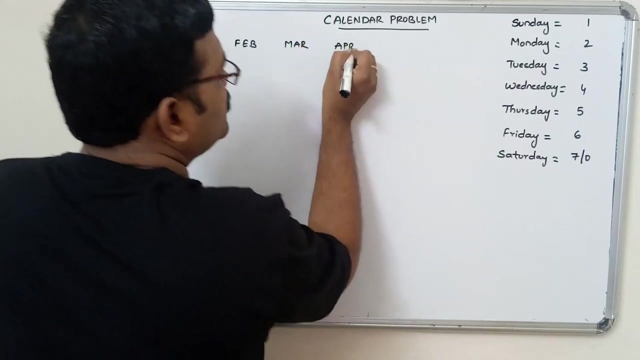 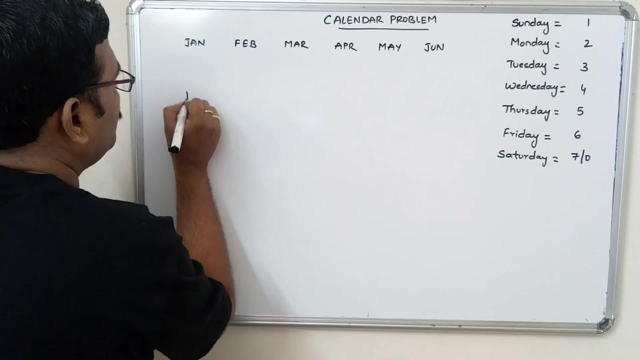 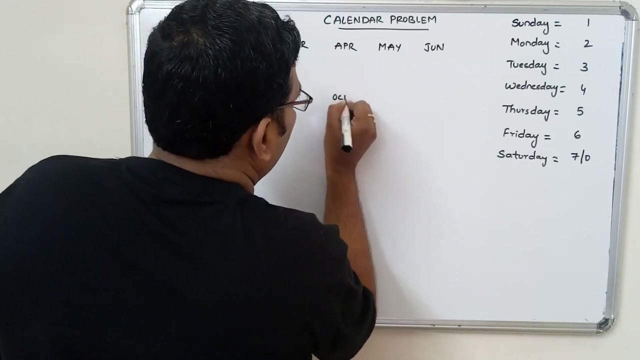 so first give the codes one, two, three, four, five, six and seven or zero. right now let us write the codes for months. write down the code for months: january, february, march, april, may. january, february, march, april, may, june, july, august, september, october, november and december. now write down the codes for: 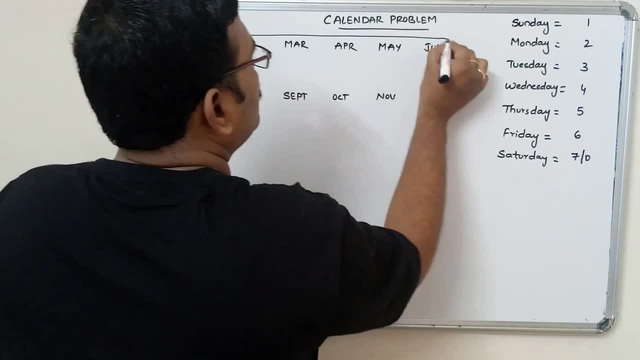 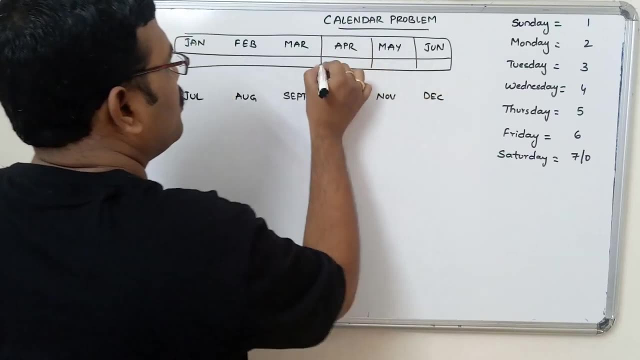 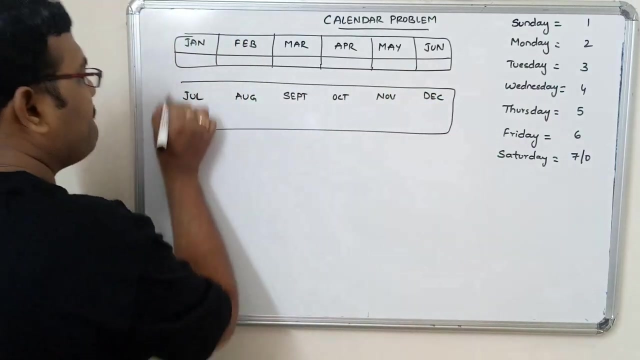 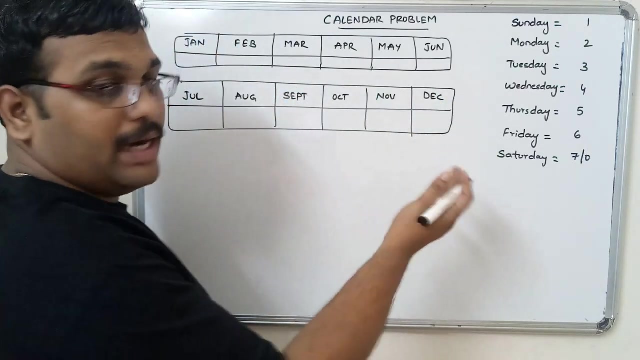 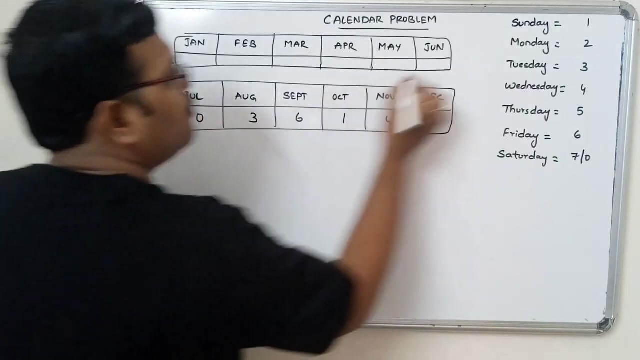 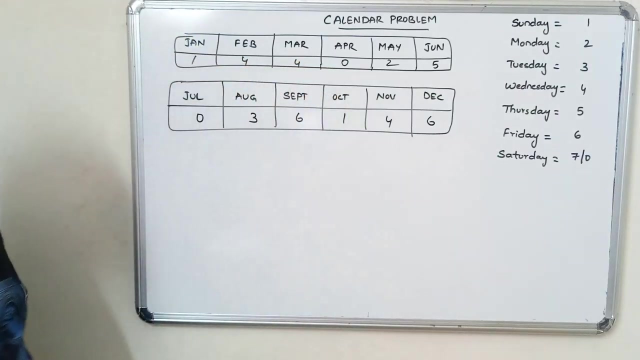 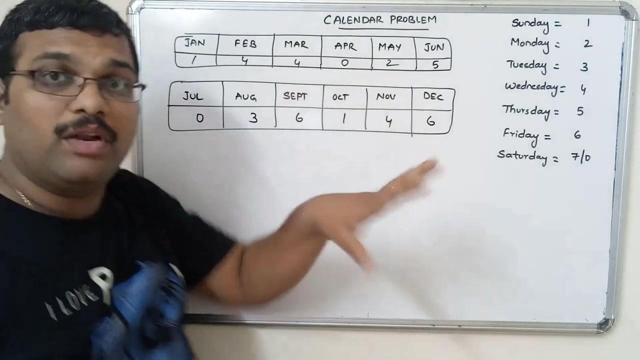 these months now. so let us start from the enigma: six four one. six three zero five. two zero four four one. these are the course given to this months. so remember, simple, just we have to remember this course. so this is very simple. just giving the order starting from Sunday. give one to the Sunday. 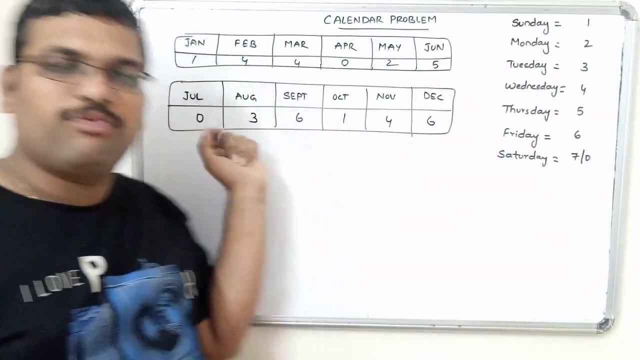 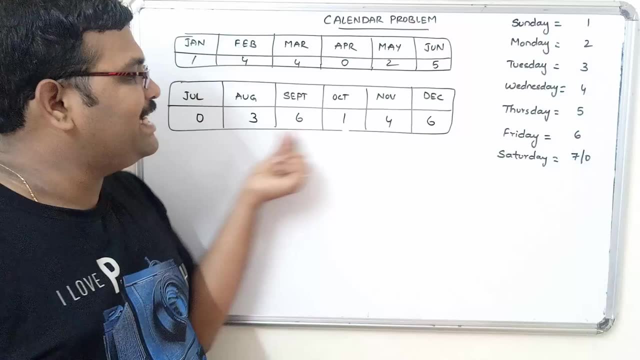 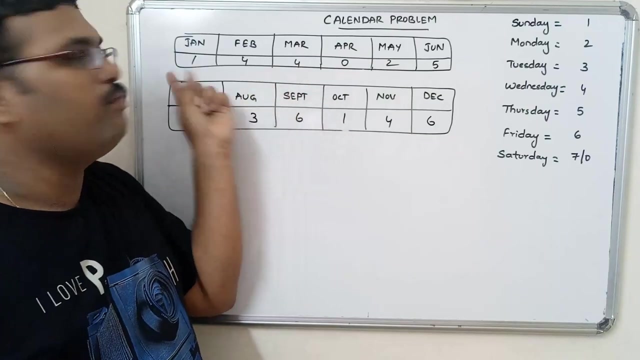 and write on the order and coming to this month. just, we have to remember this course. so just remember, like this: so one thing, a simple thing: sixty four one, sixty three, sixty four one. sixty three, zero five, two zero four and four one. hope you understood this. so it's one simple thing to 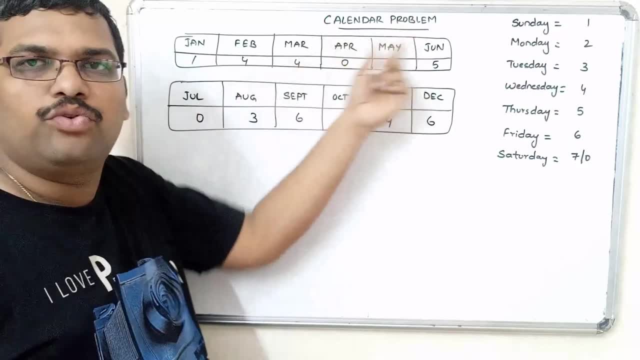 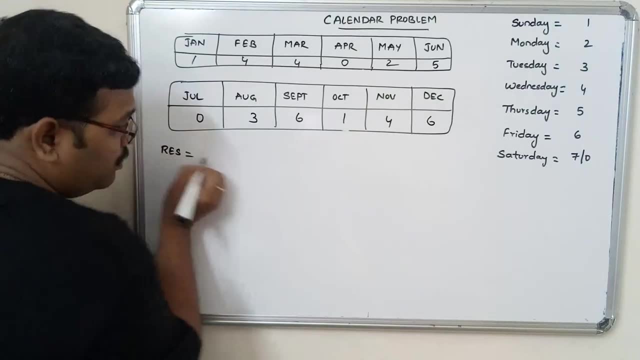 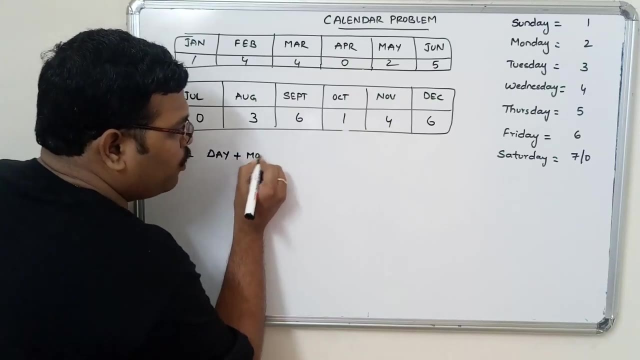 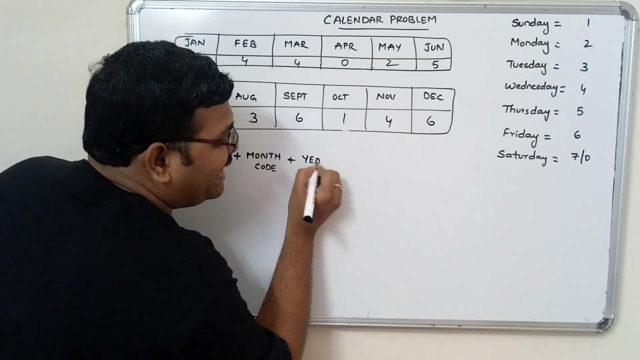 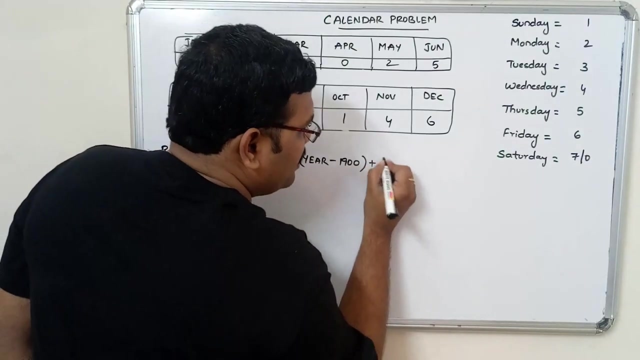 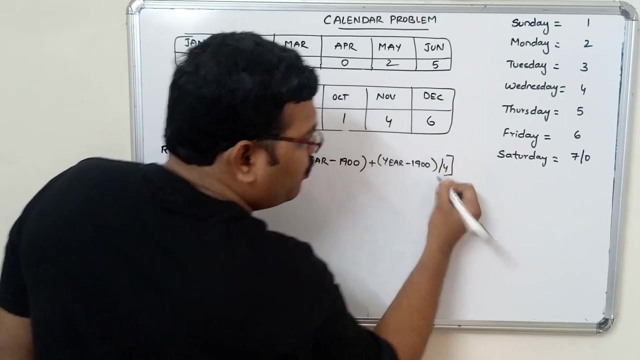 remember six, four, one, sixty three, zero, five, two, six zero four and four one. now, after remembering this thing, write on the formula: result is equal to the day from the given problem plus month code from this table, plus year from the given problem minus nineteen hundred, plus again year from the given problem minus nineteen hundred, divided by four and whole. 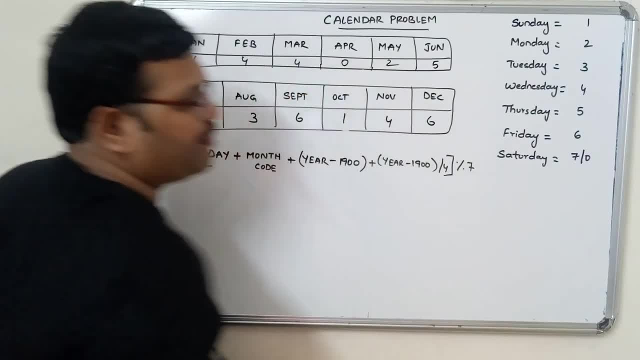 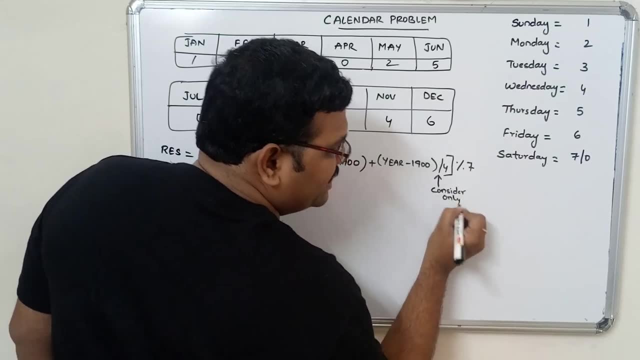 modules seven. and here in this division, consider only indikt integer part, ignore fraction, ignore fraction, even before this ideal part here over here. so by this way, we are interested in the division factor. so now we are thinking about the five Hindu unit. if you just stop, please remember that this is onesta eight, four, one, six, nine, six, eight and. 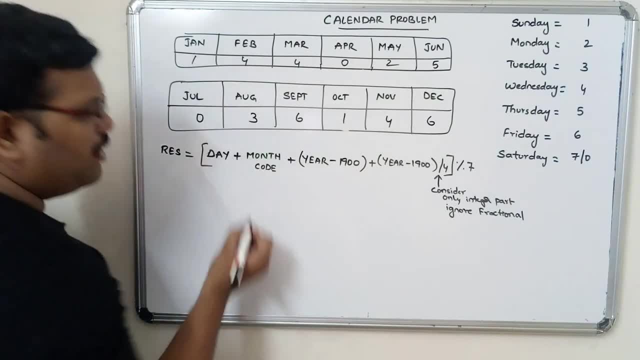 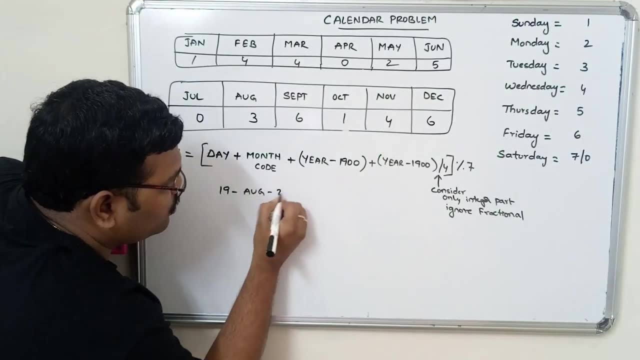 so lower down, we just will learn terms. what you learned are called Inteogens, both points and then all over. the part we cannot know is that this is only one l里. so this initial percentage, one of the three factors arevers are the three consequences, fractional, see. let us trace today's date, 19th August 2018. now, result is equal to: 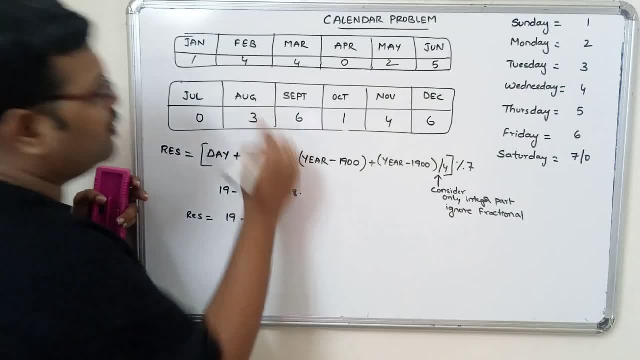 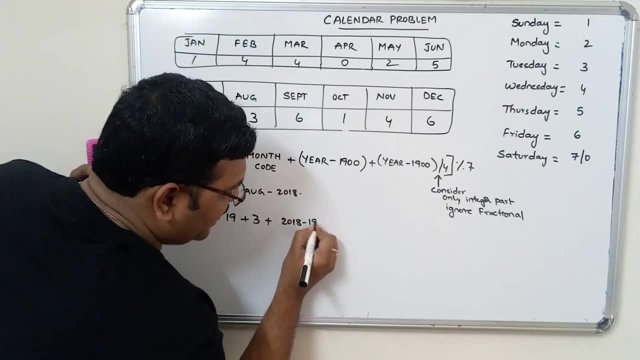 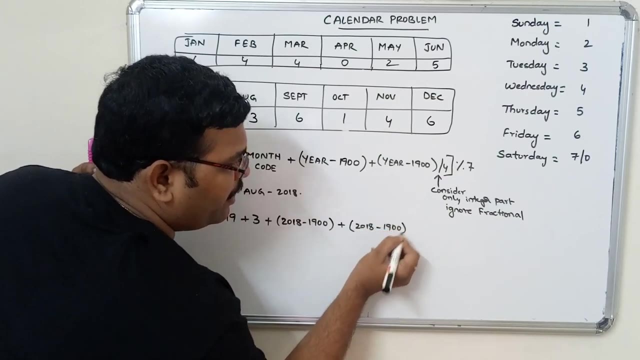 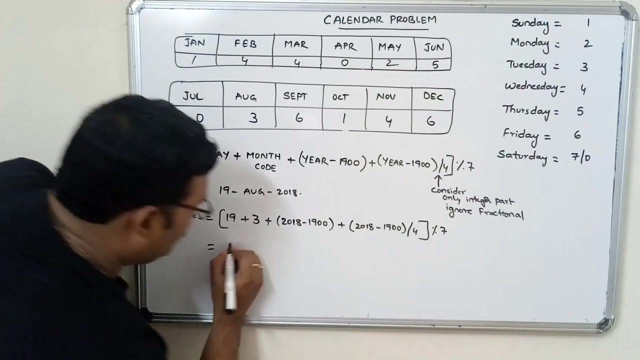 day 19 plus August. August month code is 3 plus year 2018 minus 1900, plus again 2018 minus 1900. divided by 4, whole mod 7. let us see 19 plus 3, 2 plus Fed' a. 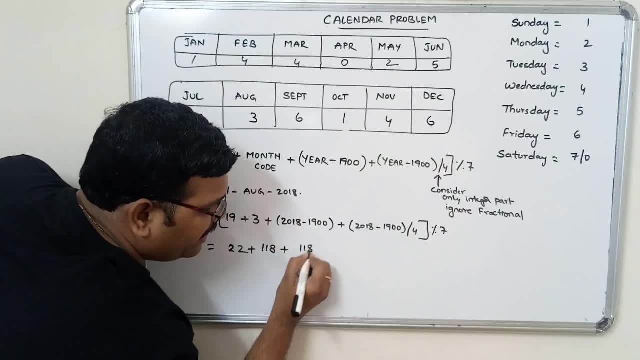 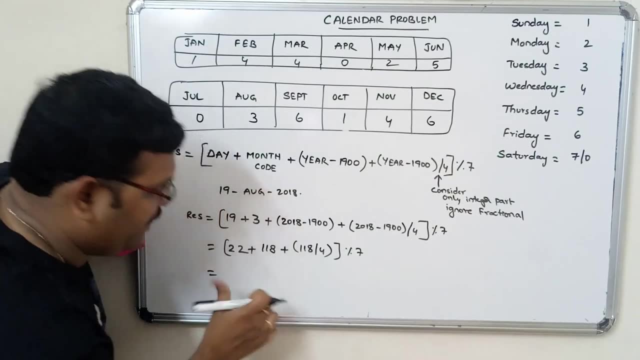 mine is 1900, 118 plus 118, divided by 4, whole mod 7, again 22 plus 118. how much so 140 plus 118, 118, 217.. 1992 cards cheese: 118 minus 1900.. What is that? 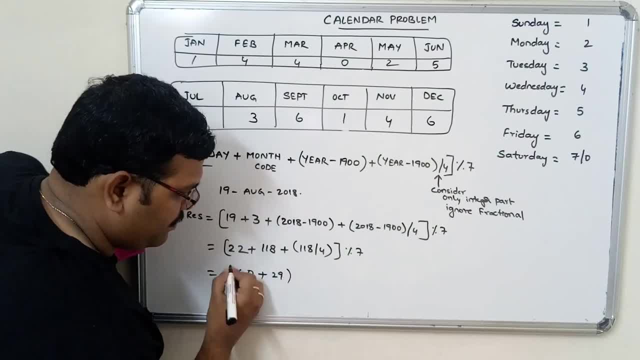 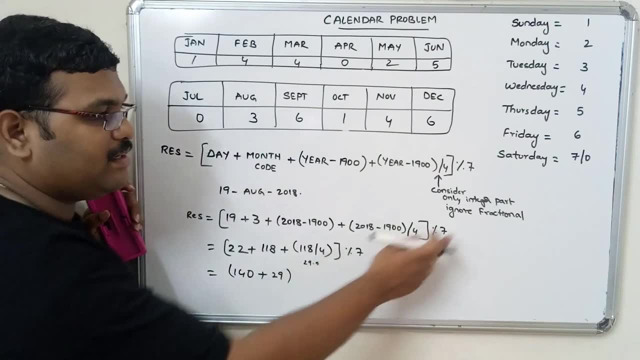 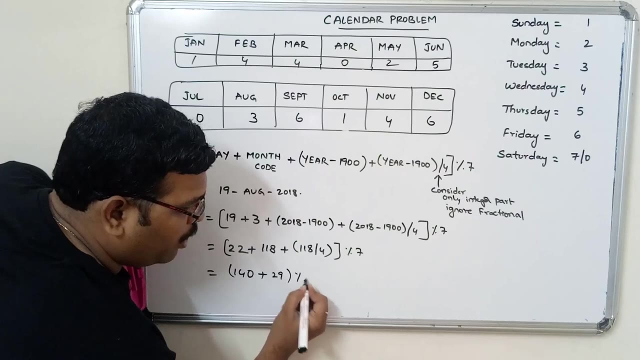 divided by 4, 29, so that is almost 29.5. so just consider only integer part, ignore the fractional part. so I will consider only 29 mod 7, that is equal to 169 mod 7. so this mod means consider the reminder after division, reminder after division. 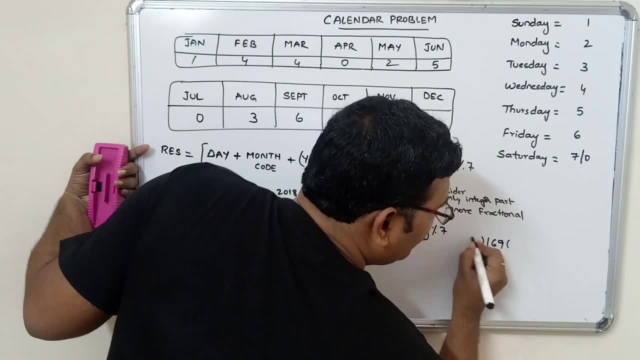 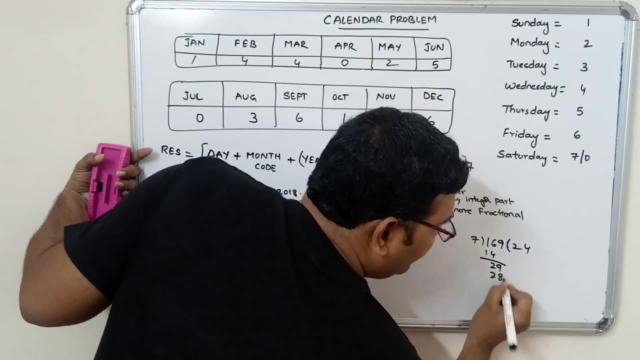 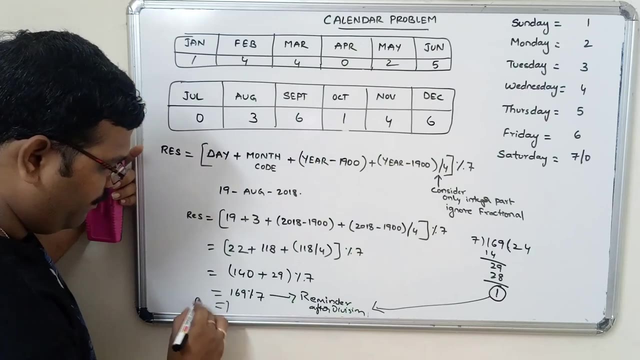 so 169 divided by 7 is 7. twos are 14, 29. so fours are 28: 1. so this is the reminder. so this will be the answer for this. so result is equal to 1. you see the result here. this is the result here. this is the result here. 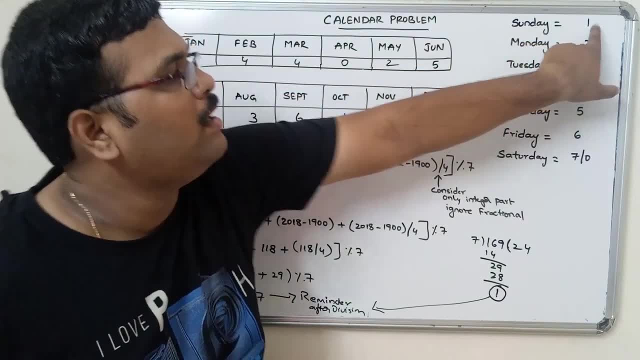 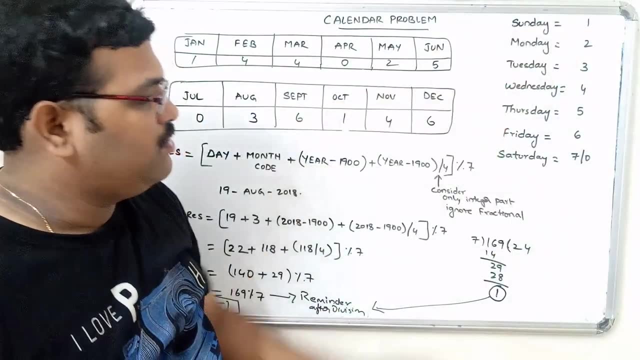 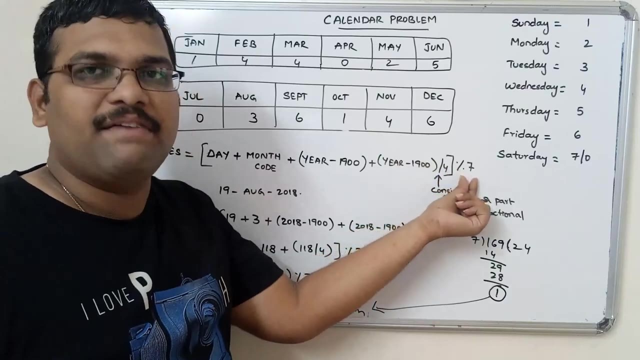 what is the day for given result? one is a Sunday, so today is a Sunday, right? hope you understood this. so day, month code: year minus 1900. year minus 1900 divided by 4 mod 7, so this gives the result in between 1 to 7. because here we are. 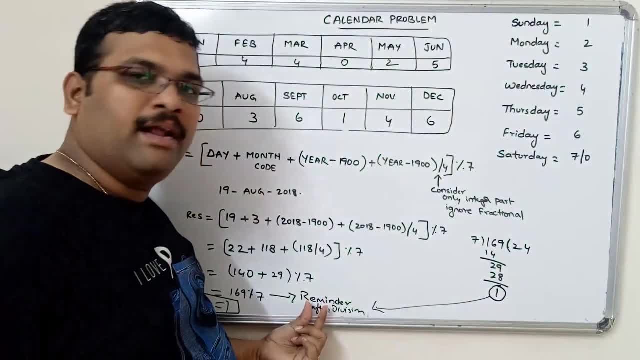 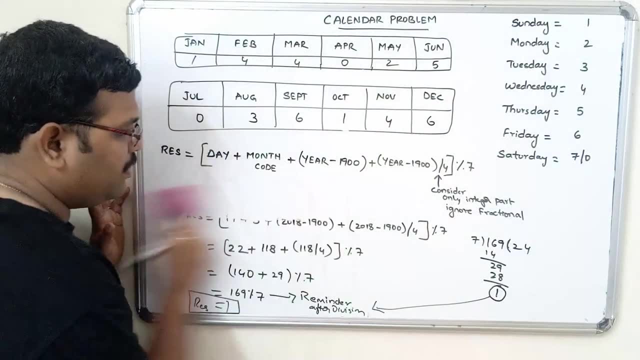 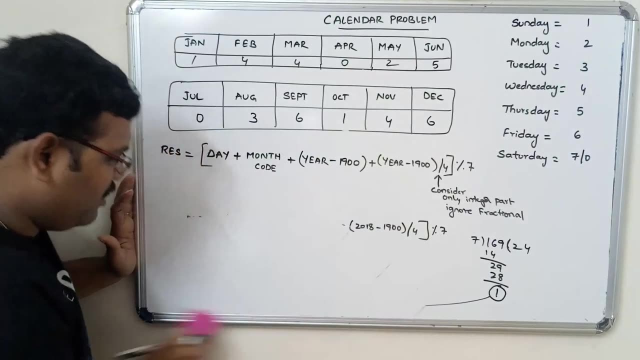 performing the mod operator. mod operator means just reminder. consider the reminder, just reminder. consider the remainder. mod operator means just reminder, reminder after performing the division. so let us take one more date and find the date. this is a very simple method, but only the difficulty is we need to. 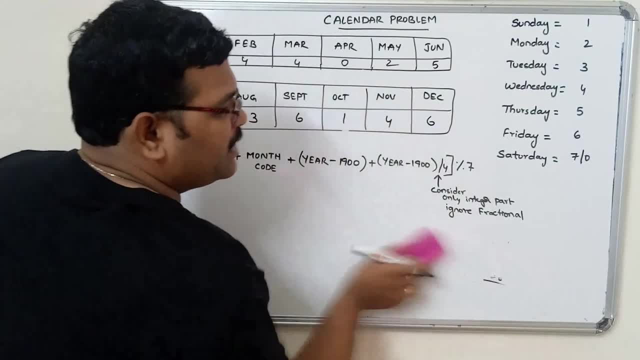 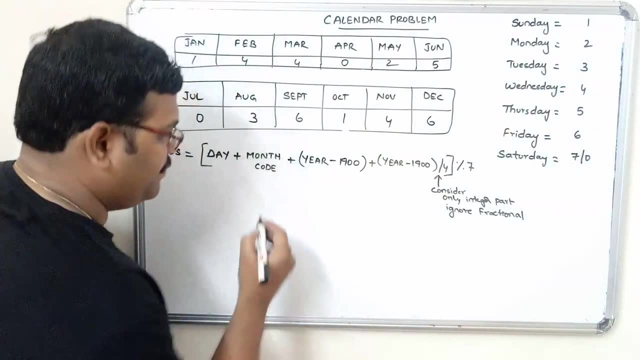 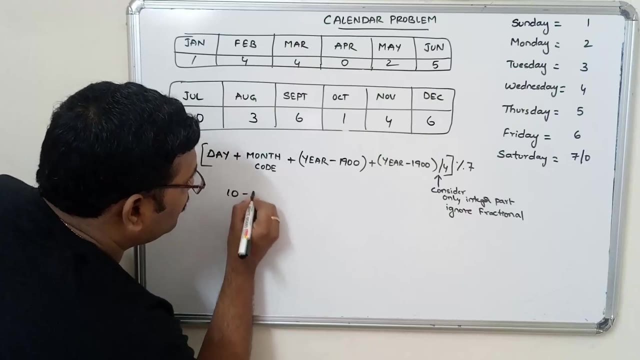 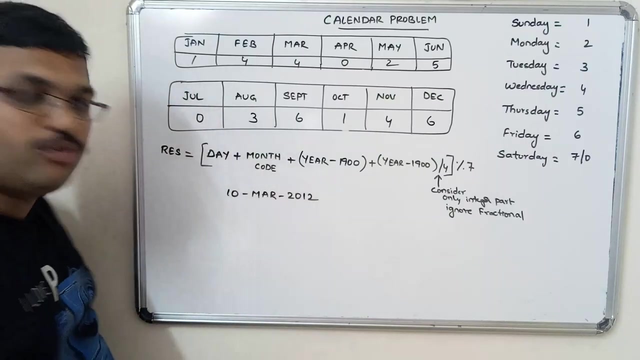 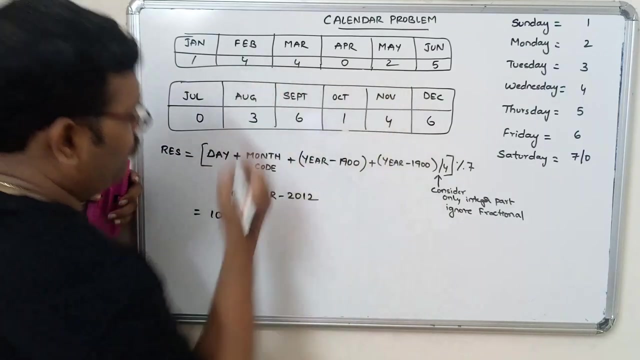 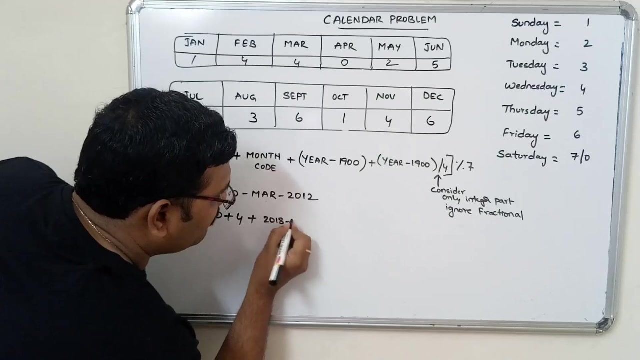 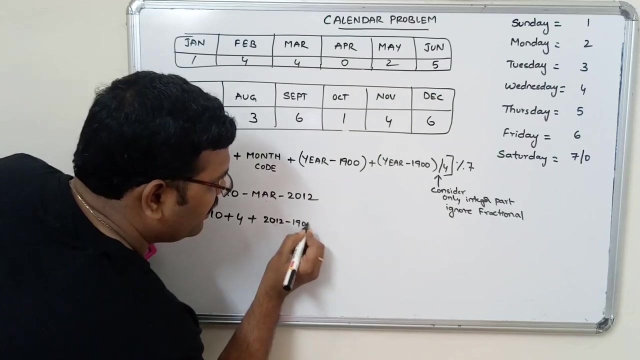 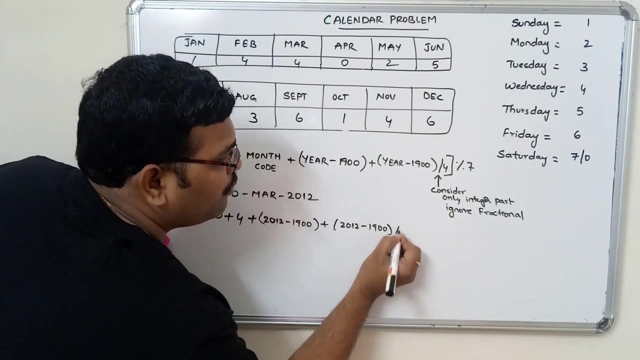 remember the month course. so if you remember this month course, automatically we can get the result right. so let us take this: 10 March 2012, 10 March 2012. so result is equal to 10 plus March 4 plus year 2018, minus sorry, 2012, minus 1900. 2012 minus 1900 divided by 4 March 7. so this: 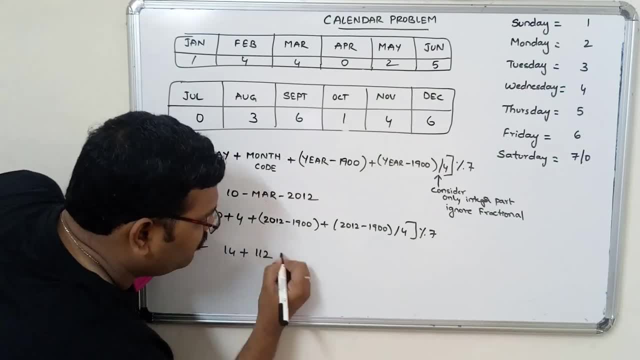 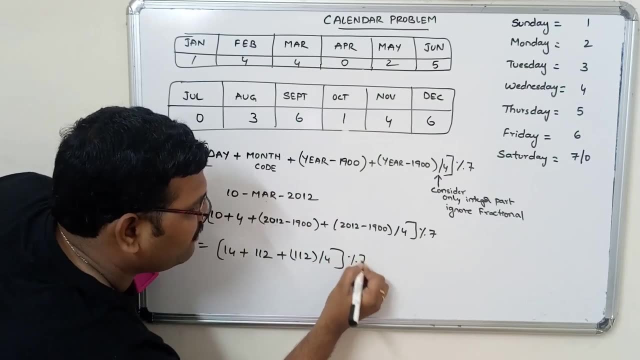 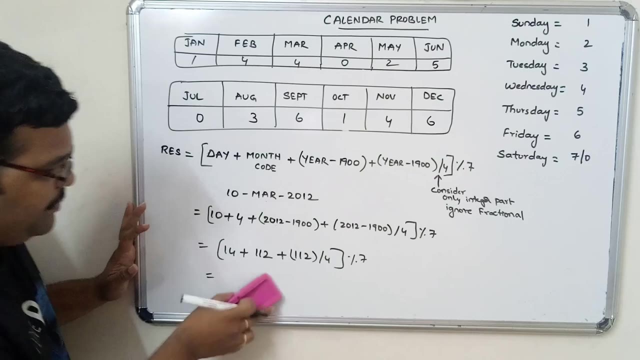 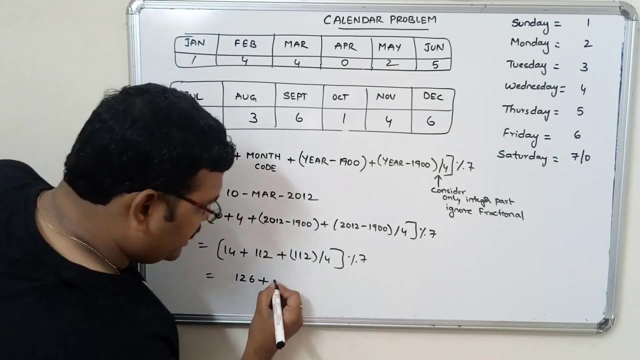 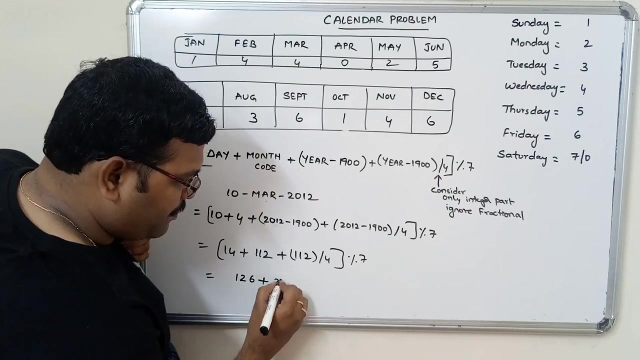 14 plus 112 plus 112 divided by 4 mod 7 right, so 14 plus 1 to all, that is 126, 1 to all, divided by 4, so 3s, so 2s are 8, 32. 32 means 8, 32 right. 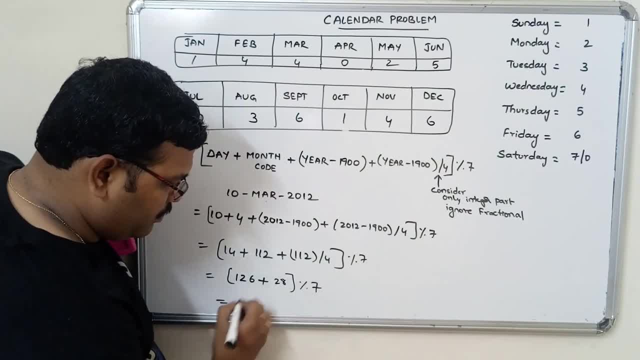 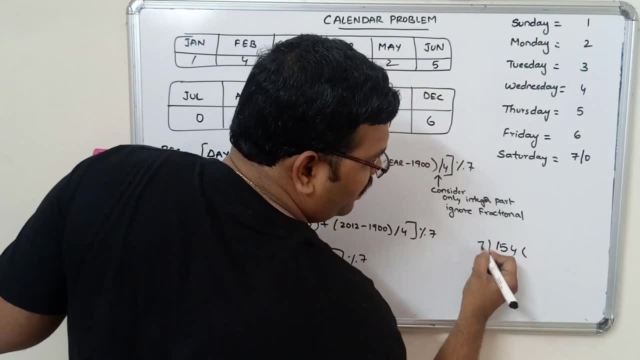 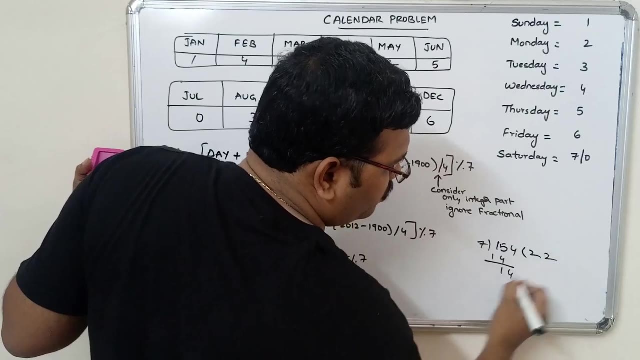 mod 7. that is equal to 154 mod 7 divided by 154 with 7. so 2s are 14. then how much? 1? 4 again 2s 14, 0, so this will be the result. so result is equal to 0. so 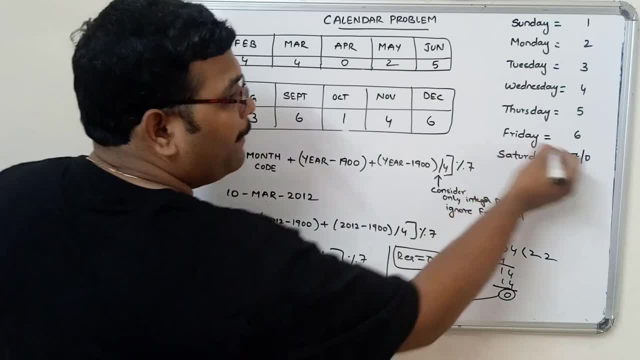 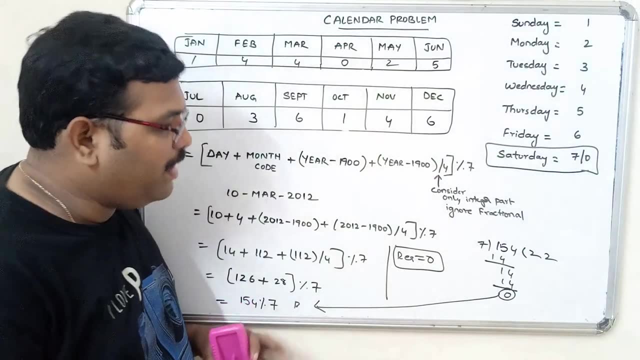 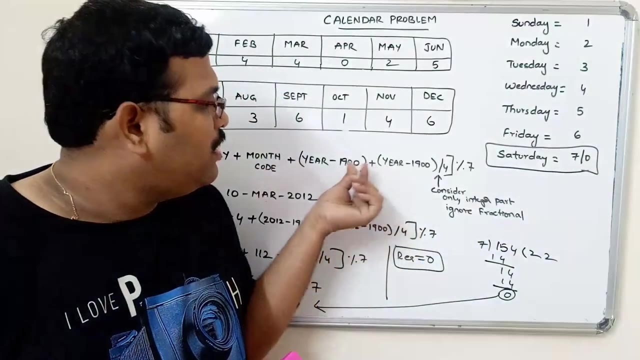 we got result is equal to 0. so what is the day? it's a Saturday, so you can find it in the calendar. we'll get the Saturday right. so this is a simple procedure to find the day for the given day and it will be acceptable if the day, if the year, is greater than. 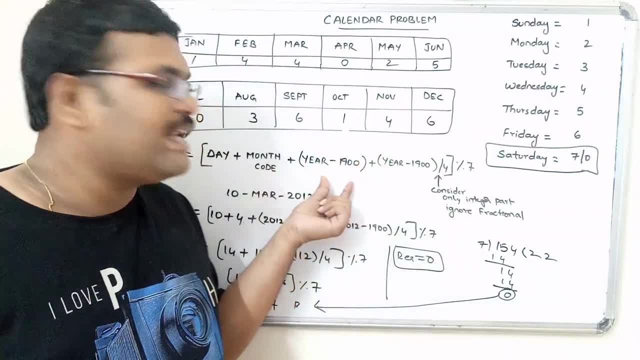 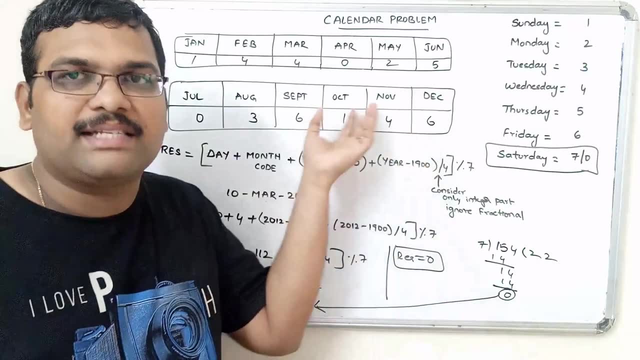 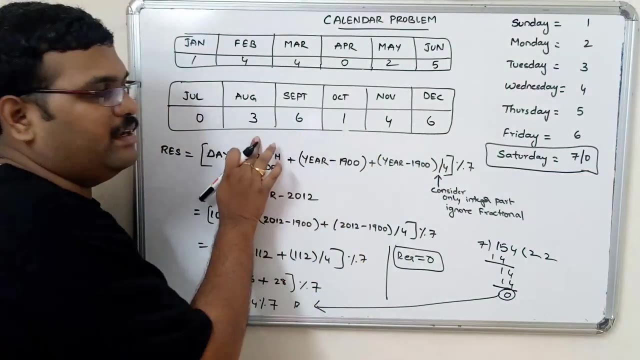 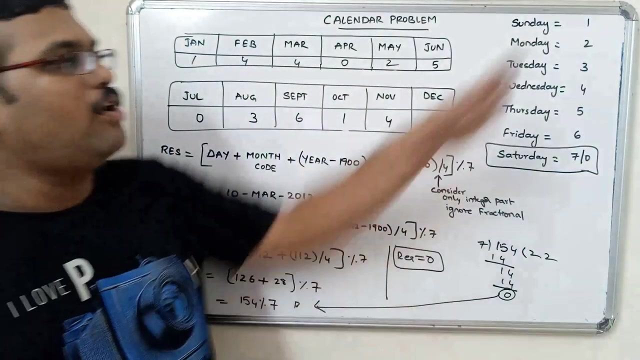 1900. we'll get the simple thing if the year is greater than 1900. so, once again, I'm just giving a small tip how to remember this course. so, from the left, from the bottom to top, write down 64 163, 0, 5, 2, 0, 4, 4, 1, and this is the order given for the days, right? so hope you.